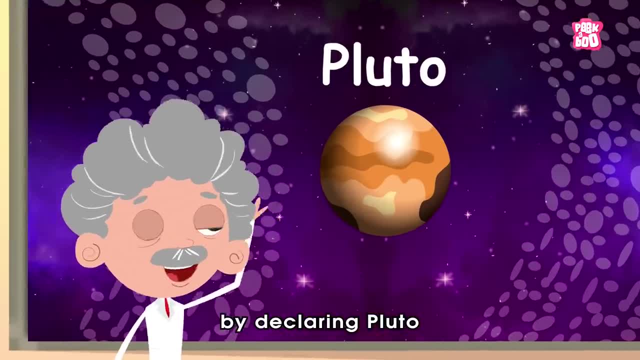 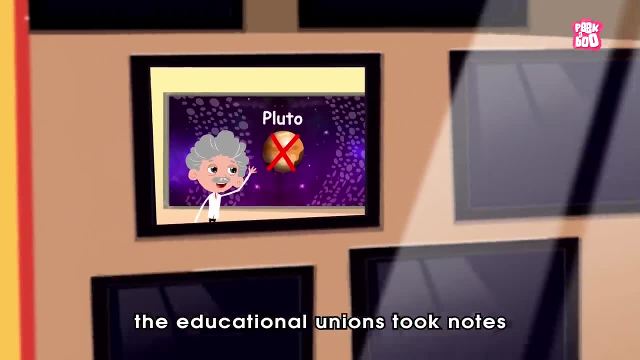 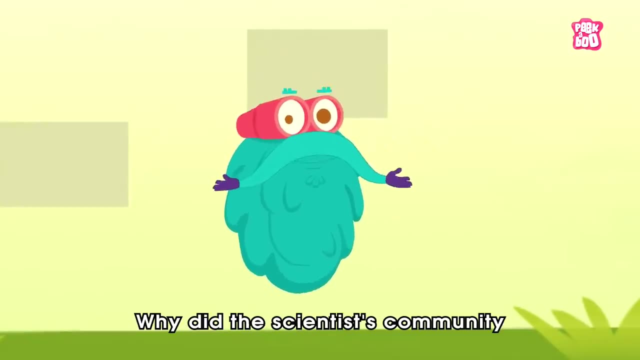 and astounded the world by declaring Pluto as not a planet. After hearing this startling news, the educational unions took notes and changed the matter in the textbooks. But the vital question is: why did the scientists' community take its title of a planet away? 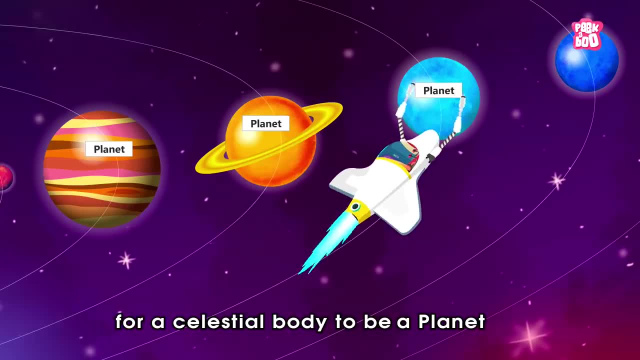 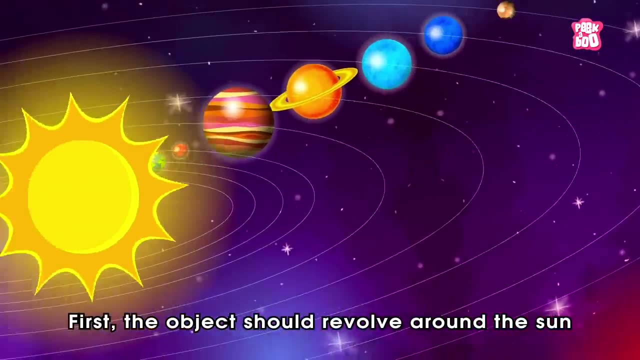 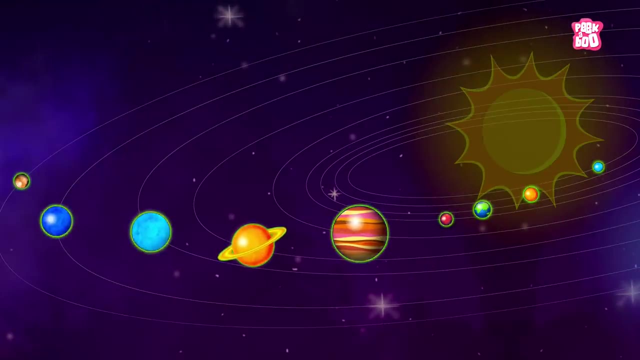 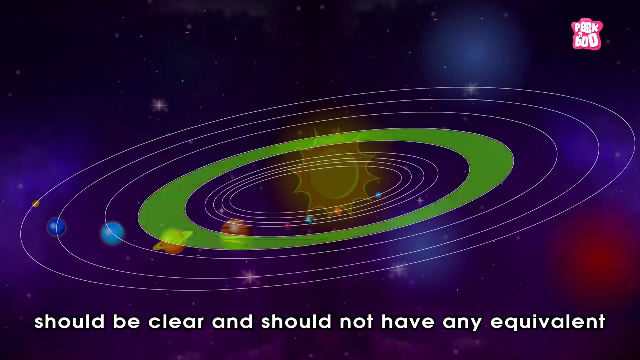 Well, according to IAU, for a celestial body to be a planet, it needs to fulfill three essential criteria: First, the object should revolve around the planet. Second, the object should be spherical in shape. And thirdly, the area around its orbit should be clear and should not have any equivalent or a bigger celestial body. 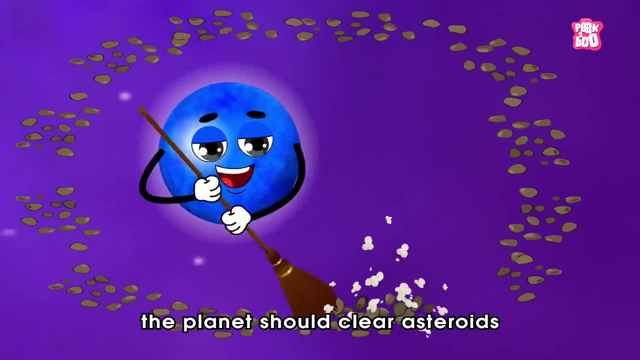 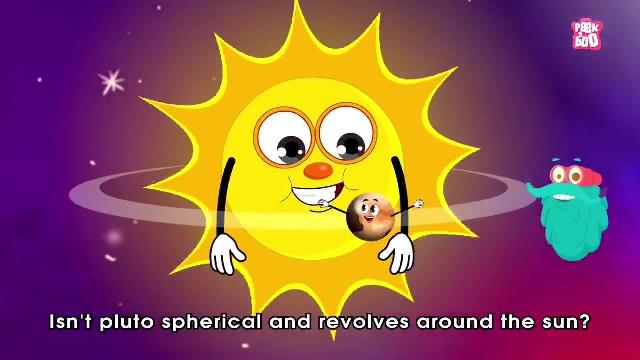 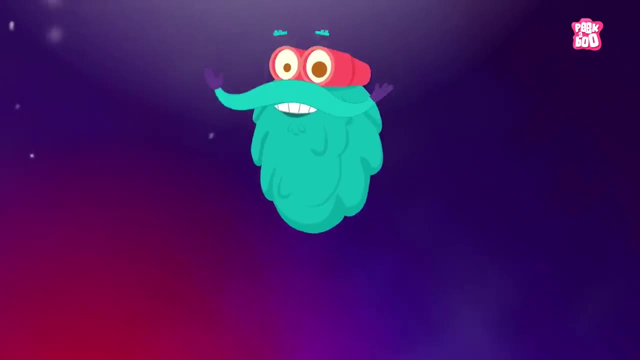 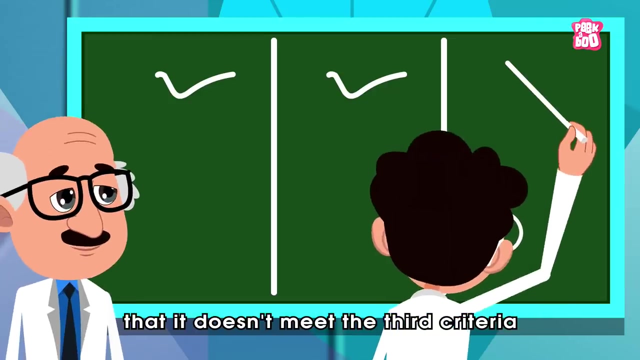 Meaning. with the help of its gravity, the planet should clear asteroids and dwarf planets out of its way. I know what you are thinking. Isn't Pluto spherical and revolves around the sun? Yes, Pluto. Pluto does fulfill these two conditions, But in the late 90s, space scientists found out that it doesn't meet the third criteria. 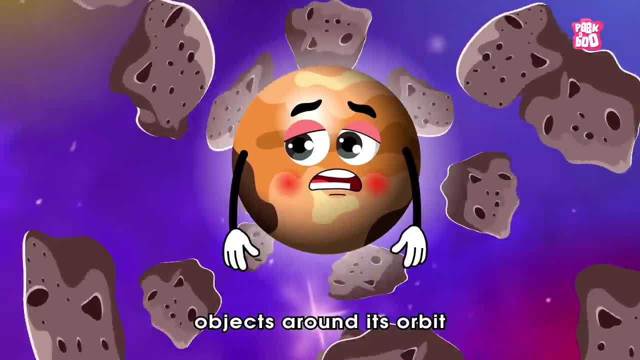 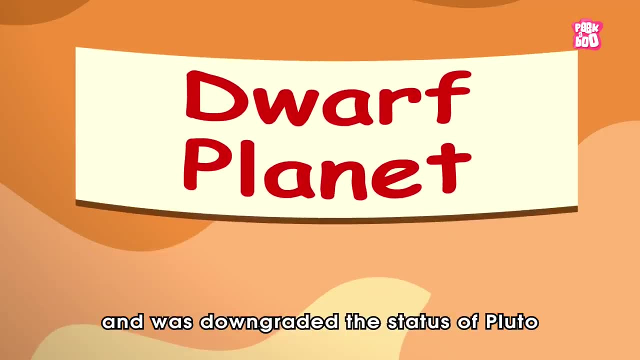 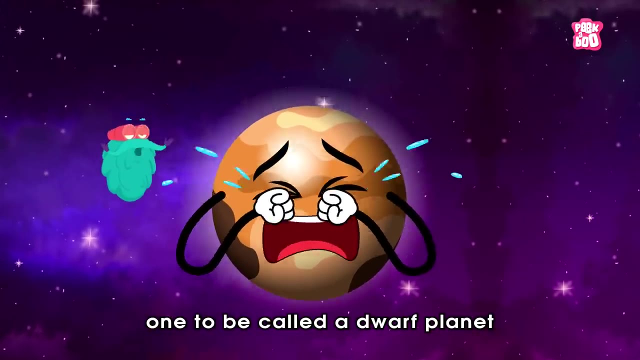 as it hasn't cleared the neighborhood objects around its orbit, because of which it can't be called a planet, and was downgraded the status of Pluto to that of a dwarf planet. But Pluto isn't the only one to be called a dwarf planet. 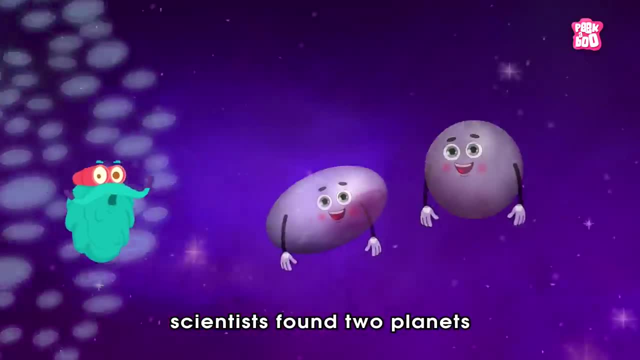 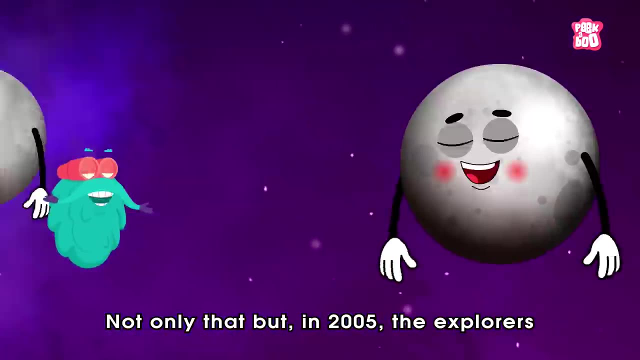 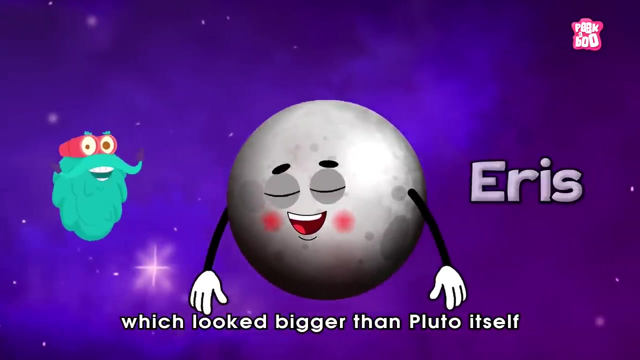 Yes, in the Kuiper belt, near Pluto, scientists found two planets, namely Homia and Makemake, which were just like Pluto. Not only that, but in 2005, the explorers also discovered Eris, which looked bigger than Pluto itself. 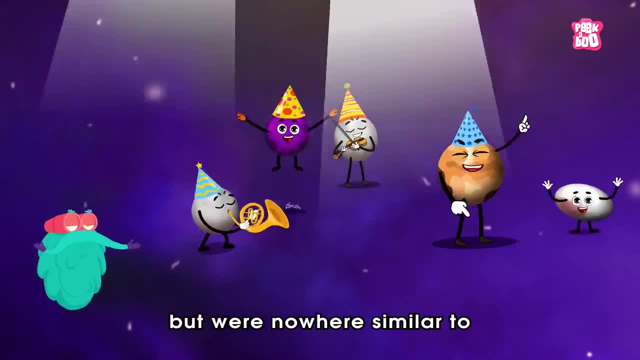 All these newly found space objects acted like Pluto, but were nowhere similar to other planets in the solar system. So that's when the IAU found out that Pluto isn't a dwarf planet. So that's when the IAU found out that Pluto isn't a dwarf planet. 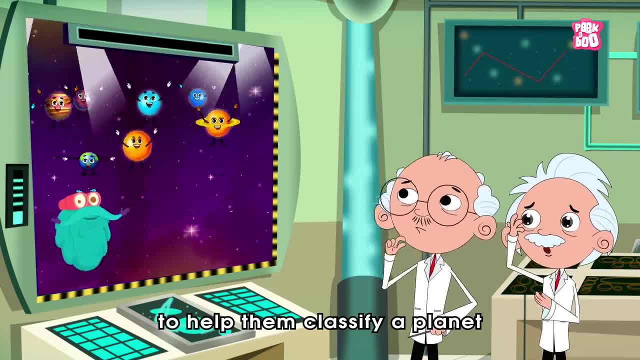 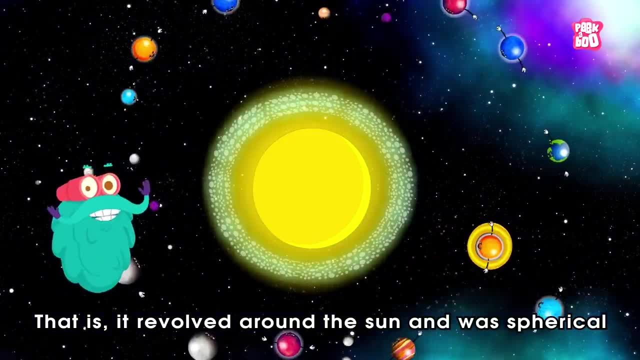 Also aboutUnadequ Tensho and Anjou. Also, we現 Ringer U, came up with a checklist to help them classify a planet and according to it, Pluto and these other planets fit into the first two criteria. That is, it revolved around the sun and was spherical.